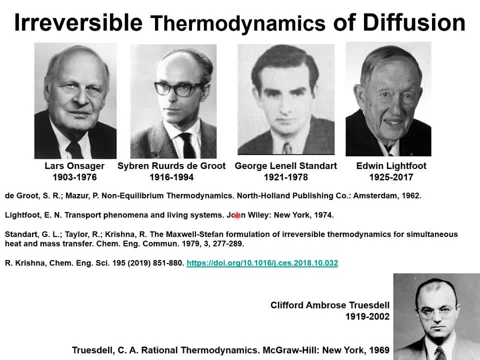 The topic for discussion today is the development of formulations to describe mixture diffusion based on the tenets of the theory of irreversible thermodynamics, also termed non-equilibrium thermodynamics. I have here portraits of four of the giants in the field of irreversible thermodynamics: Lars Onsager, who, in a seminal paper in 1945,. 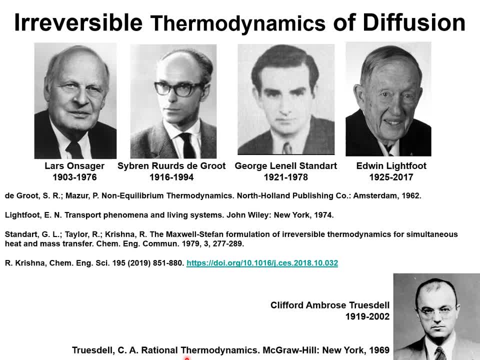 wrote. the theory of liquid diffusion is relatively undeveloped. It is a striking symptom of the common ignorance in this field that not one of the phenomenological schemes which are fit to describe the general case of diffusion is widely known. Siebren de Groot, professor of theoretical physics at the University of 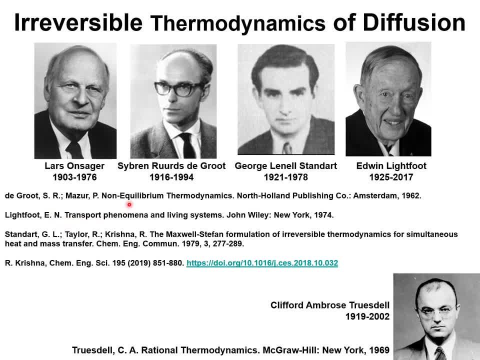